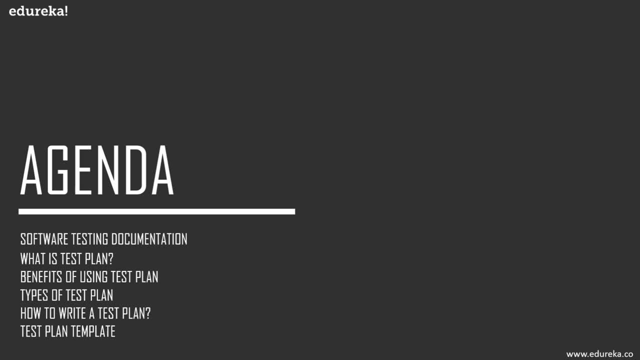 test plan and software testing. But if you guys are interested to know more about other topics in software testing or any other trending technologies, then do subscribe to our Edureka YouTube channel and learn more. So let's begin the session with a simple question. Do you guys? 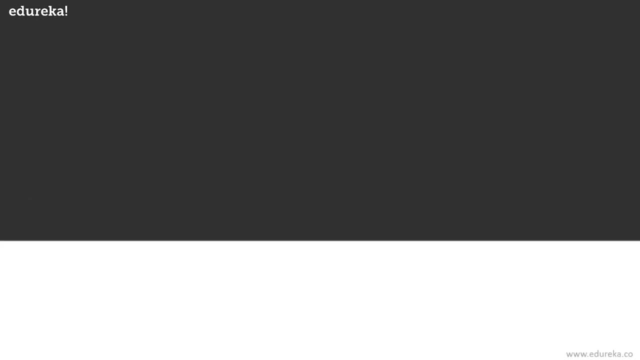 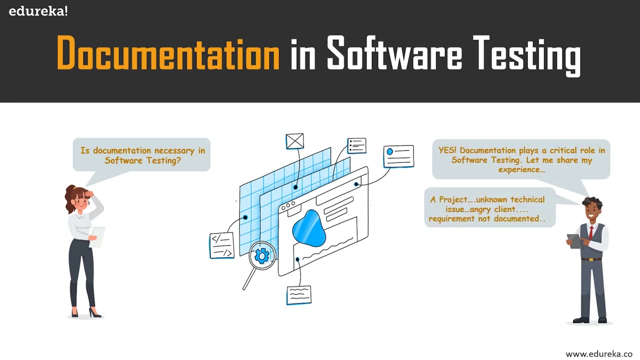 actually think documentation is really necessary in software testing. Well, yes, it is. Documentation plays a critical role in software testing. Here's a simple example to convince you people. So there's a company called, let's say, ABC. It had delivered a project with an unknown issue to one of its client, and they 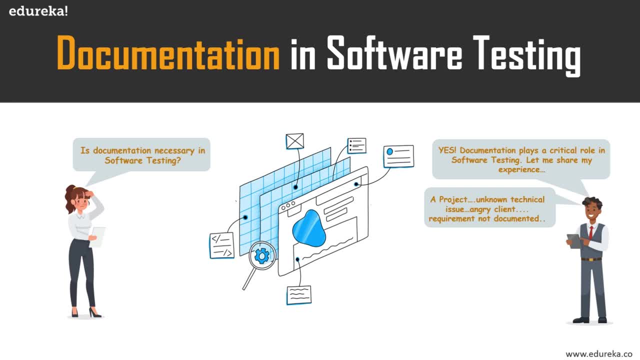 found the issue at the client side, which became a really bad situation for the company And, as usual, all the blame was put on the quality analyst of the company. So the issue was something regarding compatibility of one website with other. When this issue was taken to higher authorities, 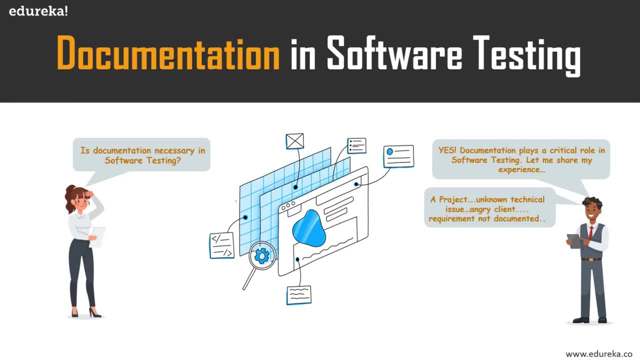 they showed the client a written proof of not receiving any such requirement, asking to check compatibility of the website also, So the issue was resolved All peacefully. In a way, documented requirements save the company from getting sued right. This example shows that just how important software project documentation really is. It can make or. 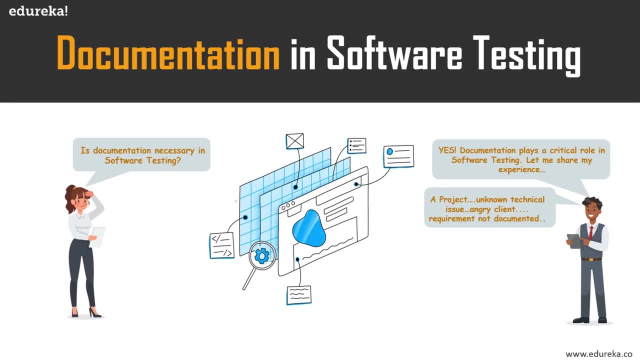 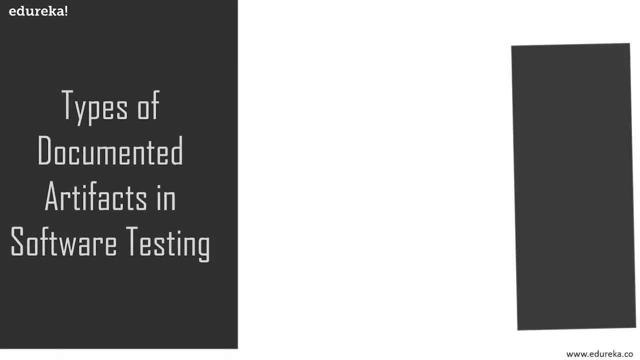 break a project, Testing should be fully documented to provide efficient resource control, monitoring and allocation. If you want to ensure your project's success, one of the most important thing is to ensure you have your project documentation in proper order. Some commonly applied documentation: 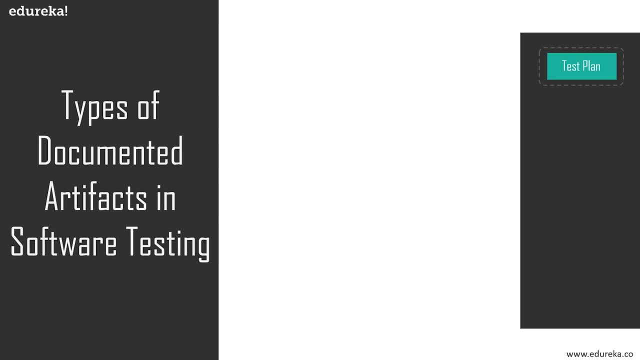 tags which are associated with software testing are. you have test plan, Then you have test case, test scenario and traceability Matrix. Let's quickly go through what each of them are. But as for today, our main concern is about test plan. So test plan is a document which is prepared at project level. 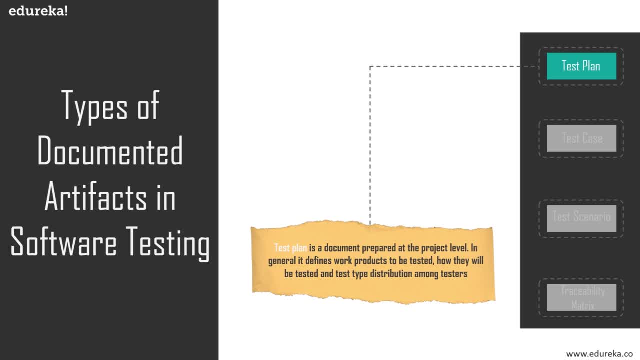 in general. It defines work products to be tested, how they'll be tested and test type distribution among testers and many other things. It also includes test environments, tools that you can use when you're testing and many of the details- Almost everything about testing- and then you have test case. test cases involved a set of steps. 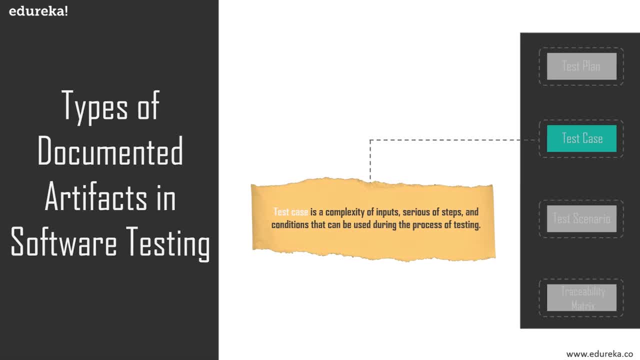 conditions and inputs that can be used while performing testing tasks. So the main purpose of writing test cases is to make sure whether a software plan passes or fails in terms of functionality and many other aspects. for the more, test cases are written to keep track of testing coverage of a product. 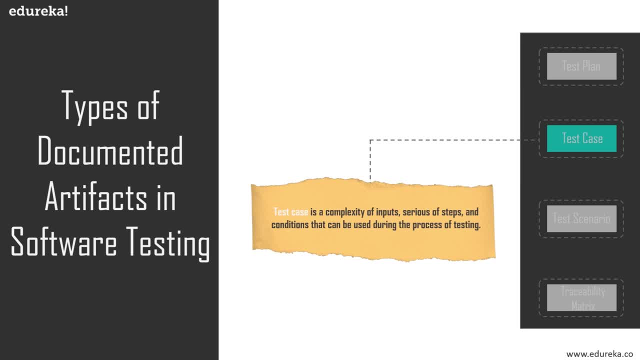 that you're testing. There are many types of test cases, such as functional negative, logical test case, physical test case, User interface test case and many others. If you want to know more about test cases, then there's a video in edureka software testing playlist. 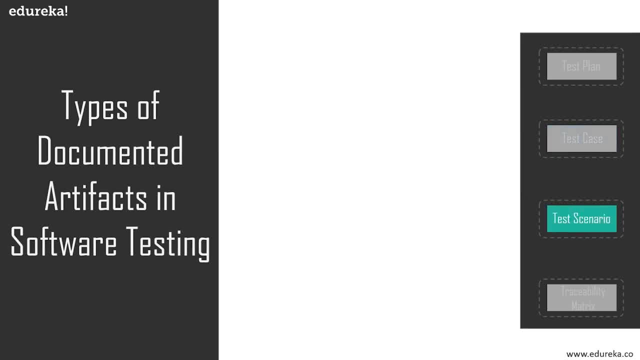 please do check out. moving on to our next type of documentation, which is test scenario, Let's see what that is Basically. a test scenario is one line statement whose main purpose is to inform which particular area of the application are you going to test test scenarios? 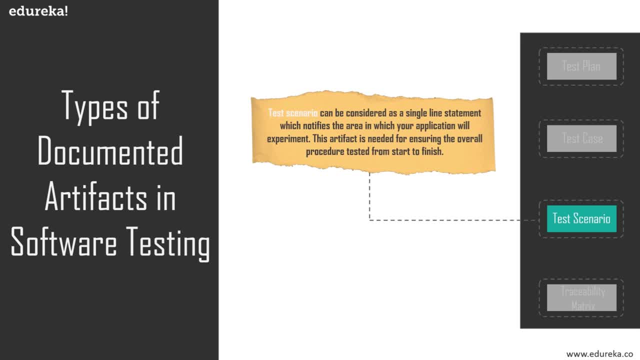 are used to ensure that all process flows are tested from end to end. For a particular area of an application, a single test scenario may be enough, but, as for others, the number may go up to a few hundred scenarios, depending on the significance and the complexity of the. 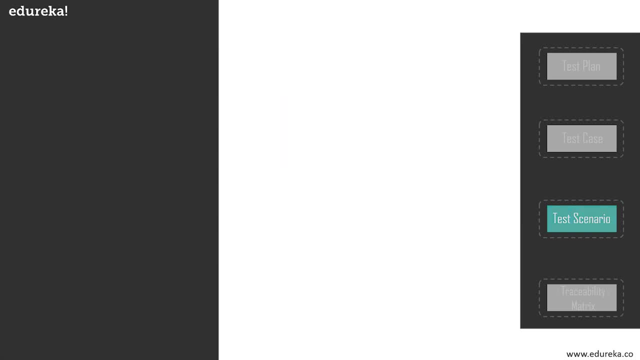 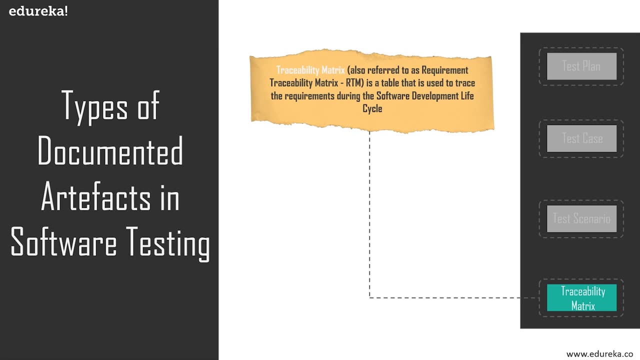 application that you're testing. So that's what a test scenario is. Then, finally, we have something called traceability Matrix. It's also referred to as requirement traceability Matrix or RTM. It's a table that is used to trace the requirements during the software development life cycle. 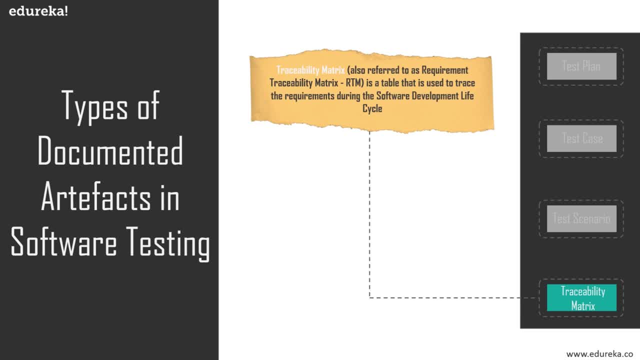 It can be applied in various usages, Like forward tracing, that is, requirements to design or coding, or backward tracing, that is, from coding to requirements. So these are some standard documentations that are used during entire software testing process. as for today's session, like I said earlier, we will be exploring test plan in detail. 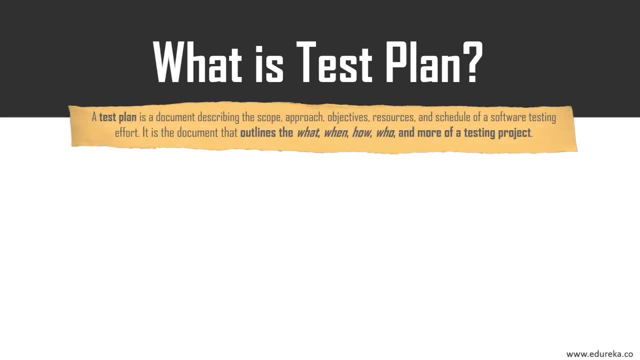 So what is a test plan? The overall software testing process also has many other formal procedures, but the plan is actually where we begin. Are there? a testing company actually begins like any project, when you have a plan in place, chances are it will go very smoother. So a test plan and software testing is the document that outlines the 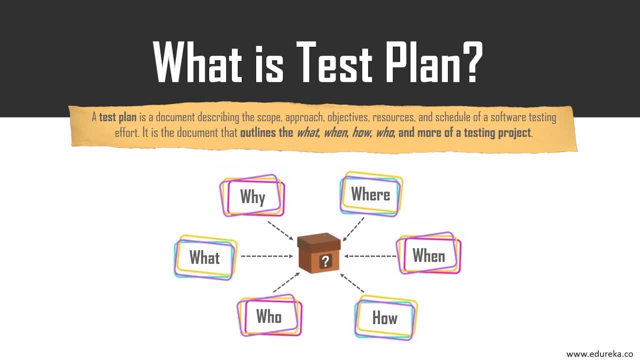 what then? how, who, and more of a testing project. Well, in general, it includes the objective and the scope of tests that are to be run. It contains guidelines for testing process, such as approach testing, task environment, needs, tools, requirements, schedule Constraint and many other things. 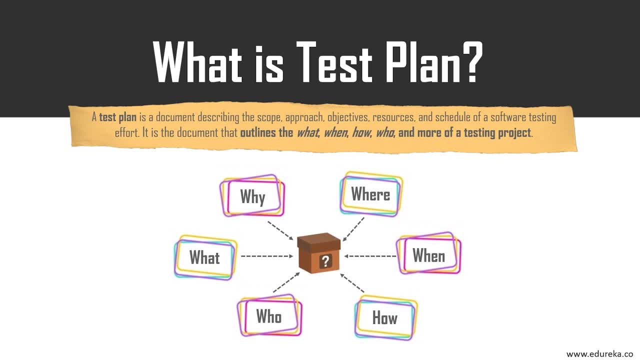 So test planning is the first thing that should happen in the software testing life cycle. It's a very important because it summarizes the testing process. The plan is basically broken down into manageable pieces so that we know how to deal with each aspect of that process and it's a record of our objectives, as in the testers objective. 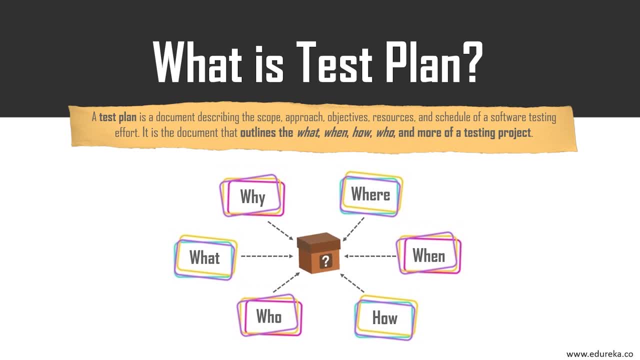 So the tester can look back and see how he actually did the testing and where he has to change. Did he follow according to the plan And all that? so a test plan essentially contains the details of what the scope of testing is, what the test items are, what the test items test or pass criteria will do and what is the need to set up the 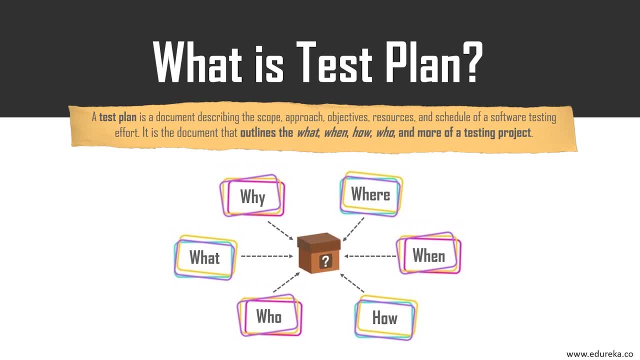 entire test environment and many other things. Well, now that I've talked so much about what a test plan is- like I said, it contains all the details before you actually start testing- you might be probably wondering: why is it necessary to invest all this time and effort to create a test plan? 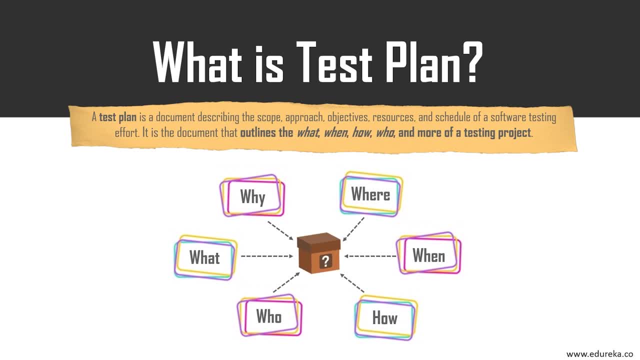 How about just jumping off to testing and getting the work started? Well, hold on, you might need to rethink. testing is an important process in software development, like cycle, which controls and determines the quality of your deliverables. So if you want to deliver a bug-free product at its plan timeline, you need a good test plan to make. 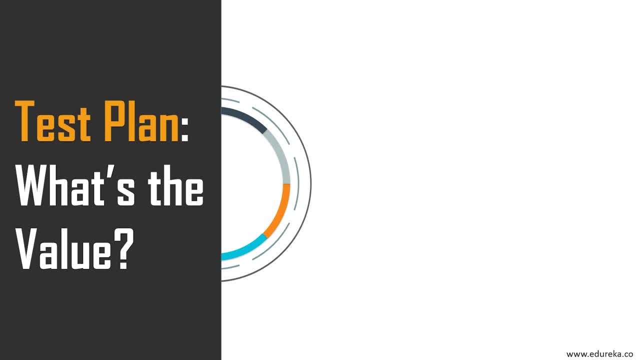 it happen. Well, here are some reasons to convince you why test plan is really beneficial before you actually start testing. So, first of all, it serves as a framework And a guide to enjoy your testing project is successful, and it will help you control risk as well. 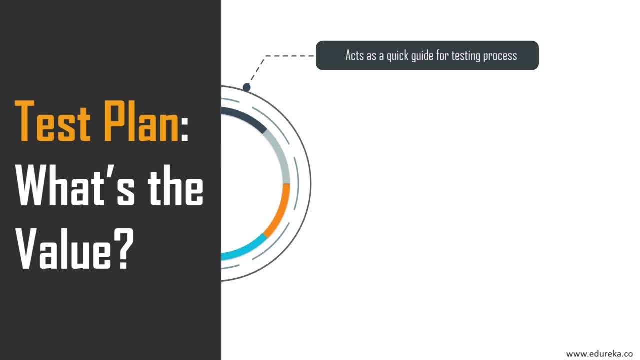 The very act of writing helps us think through things in a way We might actually not consider normally. not just in software testing, It's the case even when you plan anything in your life, right? So, yeah, the test plan contains details of testing scope, which prevents testing team from putting 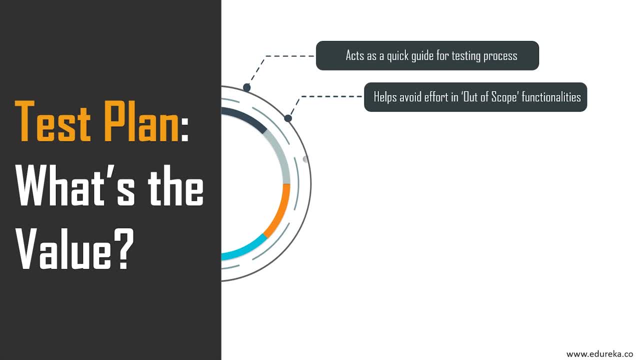 any efforts in testing out of scope functionalities. with test plan You can have rough estimate of time and effort which is needed to complete the software project. It clearly defines roles and responsibilities of every team member, So every individual in the testing team knows what he is required to do. 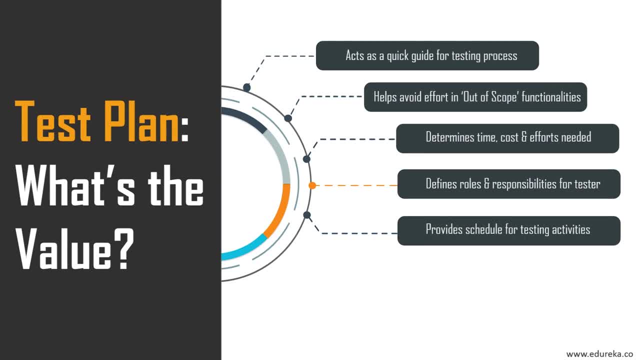 and what is expected to do. Also, it provides schedule for testing activities. Hence It provides you a baseline schedule to control and track your team's testing process. But one thing is: as changes to the test planner made, the test plan document should be updated. 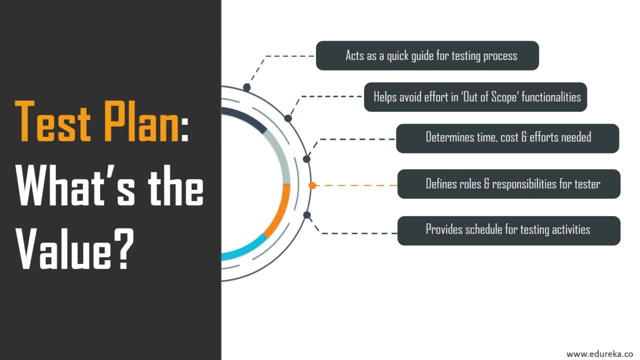 to reflect the new decisions that you have actually made. So test plan is not some a fixed document or something. It keeps changing according to the requirements and the test process that you follow. it also outlines the resource requirements and equipment needed which are essential to carry out the basic testing process. 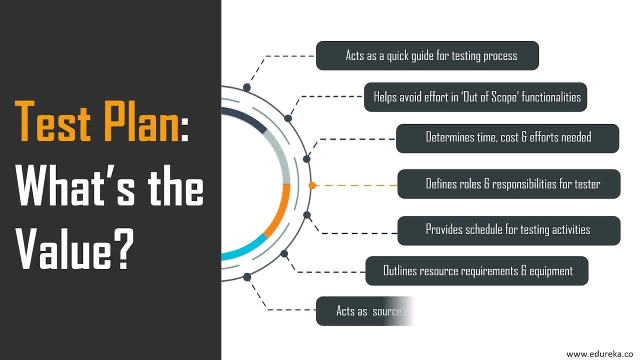 So it guidelines the testers, thinking it acts as a source of proof if you need to refer to anything in future, just like the example which we discussed in the beginning of the company ABC. like the client had an issue, but then the client didn't specify the requirement when he was listing out his requirements. 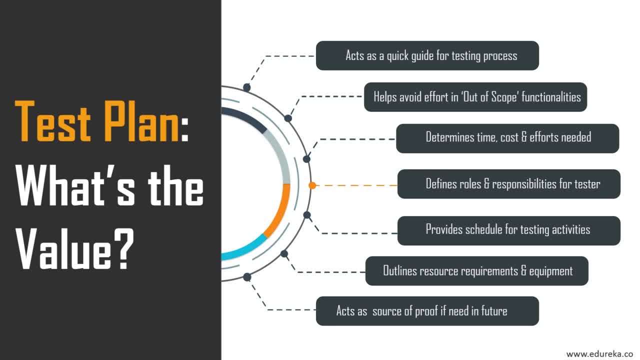 the company had proof, So somehow they were saved from getting sued. So basically it's a proof which you might refer to or which you can refer to in future. So apart from that, it encourages better communication. the test planning in the plan itself It serves as a vehicle for communication with the other project team members. 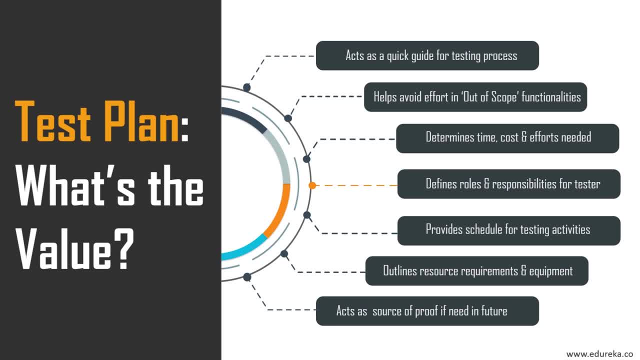 such as testers, peers, managers and other stakeholders. It also helps people outside the test scene, such as developers, business managers, customers, understand the details of testing. So that's how important a test plan is. in this way, It serves as a guide book for entire trusting process. 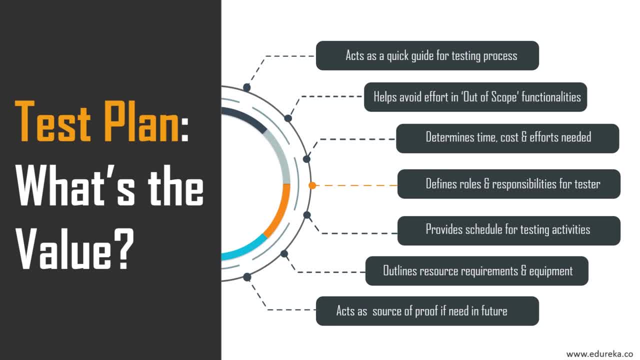 Even though we are aware of the benefits of having a test plan, We also know that testers may choose not to write one, arguing for reasons like it takes a lot of time. So, even though we are aware of the benefits of having a test plan, 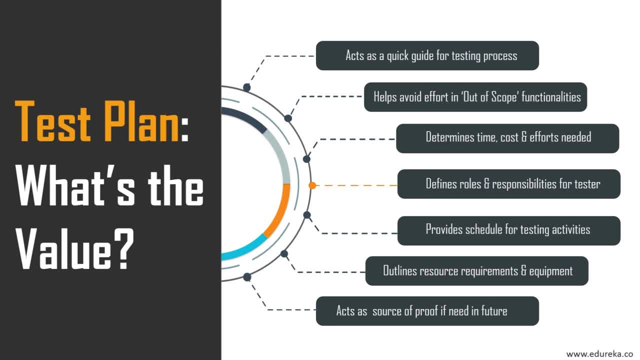 we also know that some testers may choose not to write one for multiple reasons. like it takes a lot of time and effort to prepare a very lengthy And detailed test plan, changing management in the test plan can be challenging for dynamic projects in that plan often has written information. 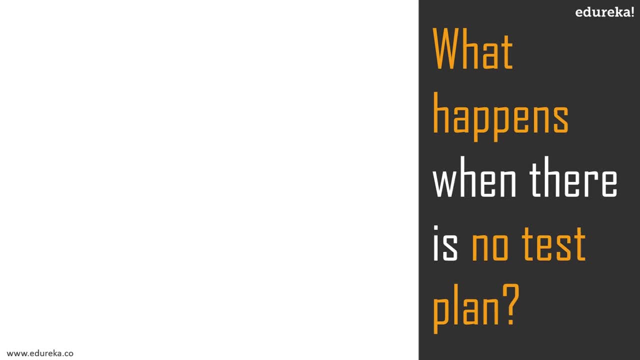 and many other reasons. So what happens when one doesn't have a test plan? Let's check out first of all. it creates a misunderstanding about roles and responsibilities. when there are no clearly defined roles and responsibilities, It could lead to important tasks of testing being left undone. 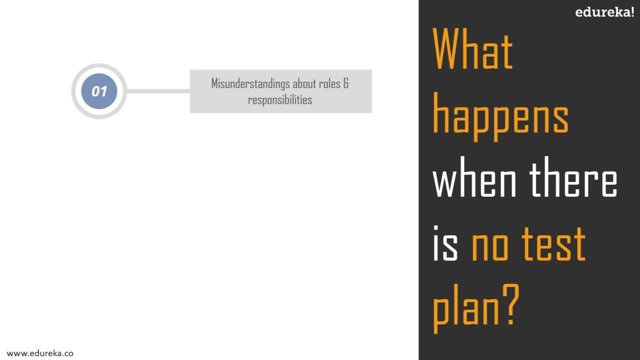 or to an unnecessary effort, For example when two testers work on the same task. So basically both of the testers are think that they have to test the product, but this testing the same feature of the product and it's just waste of time. So there's a misunderstanding about roles and responsibilities. 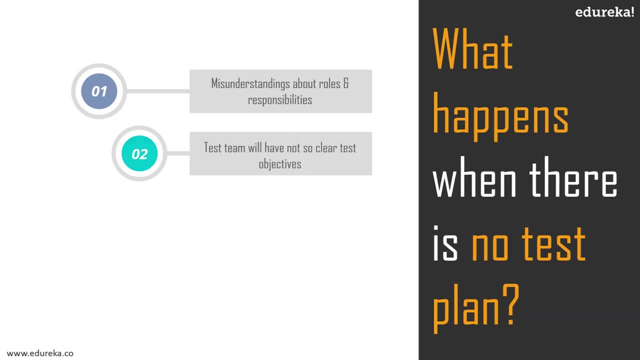 Secondly, the test team does not have clear test objectives. For example, the test team is unaware of the different types of testing that should be done on a system, as well as the reasons for doing the different types of tests without your objective for running test. 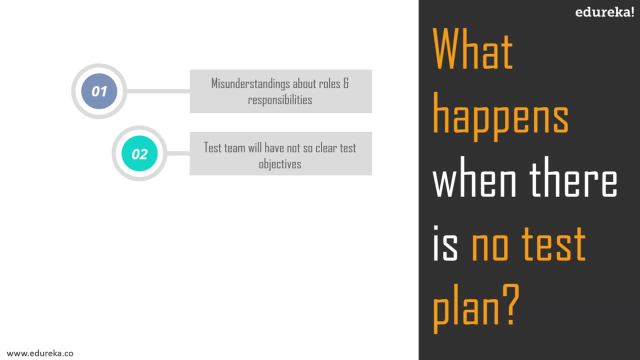 There's an increased likelihood that critical and essential system characteristics will not be adequately or properly tested. Well, again, it's a huge loss for the company and testers. without a test plan doesn't know when the process actually ends because the exit criteria is not being specified. 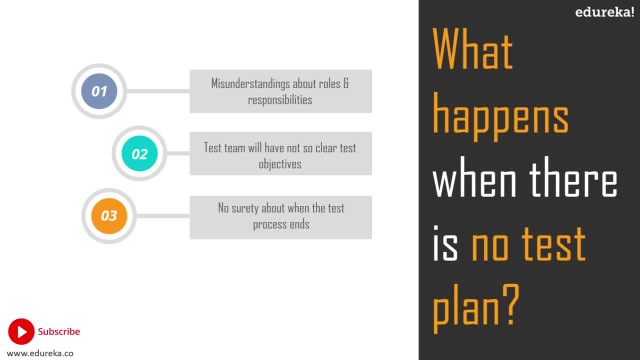 The testing team does not know when the software testing process actually ends. This is essential, as in the testing should know when the process ends because it helps to finish the task within the stipulated deadline without compromising the quality, functionality and efficiency Of the software. 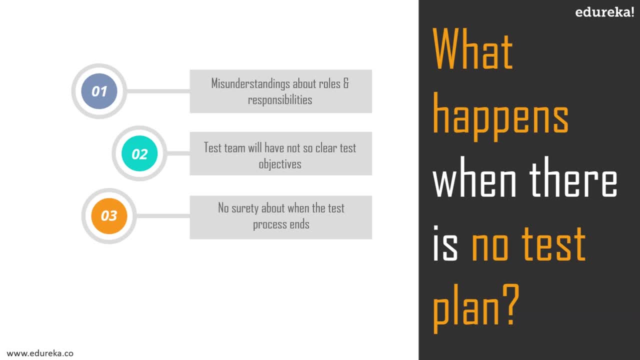 So, basically, without a proper test plan, the test team or any tester doesn't know when the software testing process actually ends and what are the proper timelines, schedule and all that, and lastly, testing scope is not defined. This is important, since the client have false expectations. 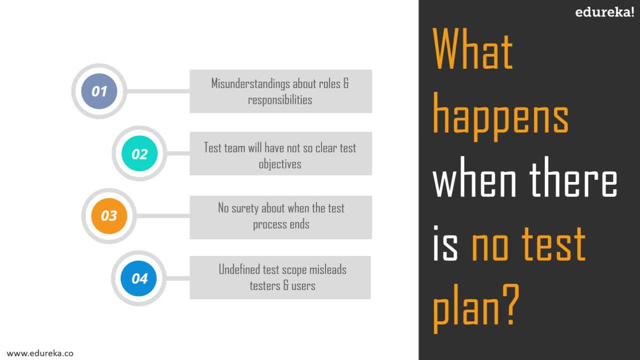 regarding the amount of testing work that has to be done and the test items that are out of scope, which should not be tested. So, due to these reasons, you need to understand that writing a test plan, or developing one, is really important task, because before you actually begin with testing, 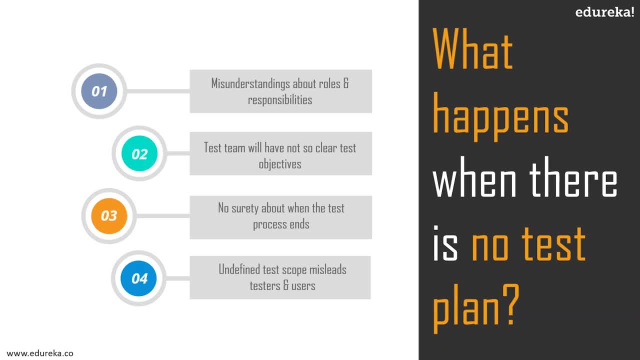 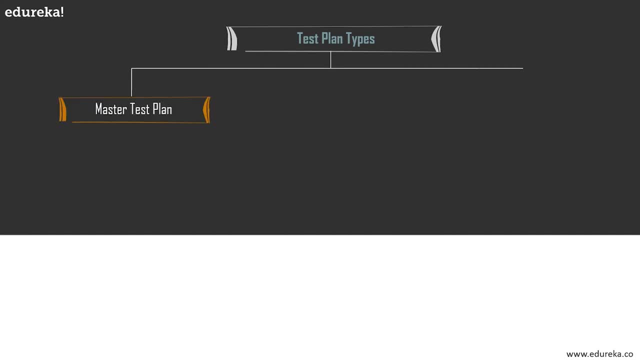 as you can clearly see, writing a test plan is more advantages than disadvantages. Well, there are different types of test plans. Let's check what they are. So basically, first you have a master test plan. It's a single high-level test plan for entire product. 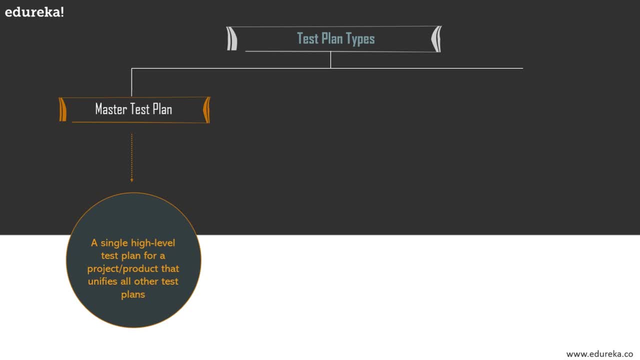 or the software project that you're working on and you unifies are. it's a combination of all the test plans, as you can see the word master right in the name. So basically it's a combination of the my new test plans which you create along the process of testing. 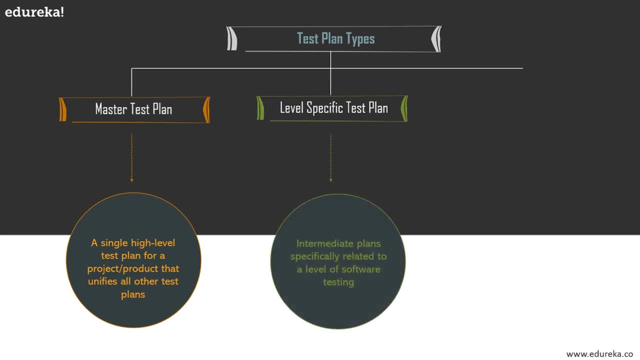 then you have something called level specific test plan. I might have discussed in previous session that the software testing has different levels, especially for important levels like unit testing, integration testing, acceptance testing and system testing. Well, not in the same order, but anyway, so you can write a separate test plan. 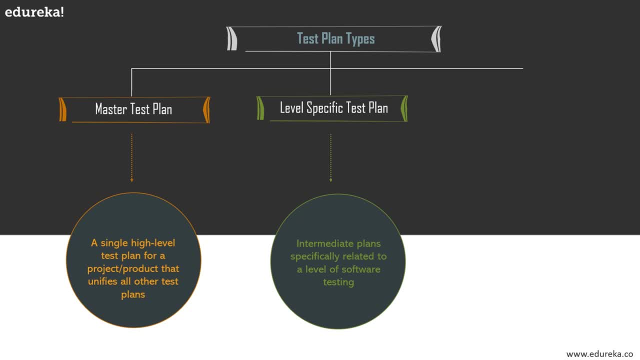 for each of these levels and when you do that, that's what we call a level specific test plan. and then comes type specific test plan. as you already know, there are multiple types of software Testing. basically having a single test plan for different type makes it complex. 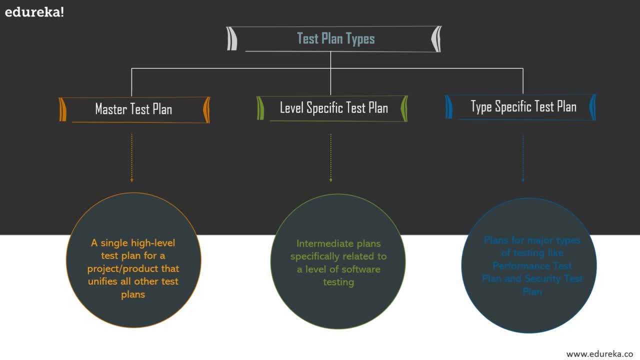 I mean it doesn't put out the benefits of test plan actually. so to make the entire process easier, you create separate plan for different types of testing that you're employing while you're testing the product, so that we call a type specific test plan this type specific. 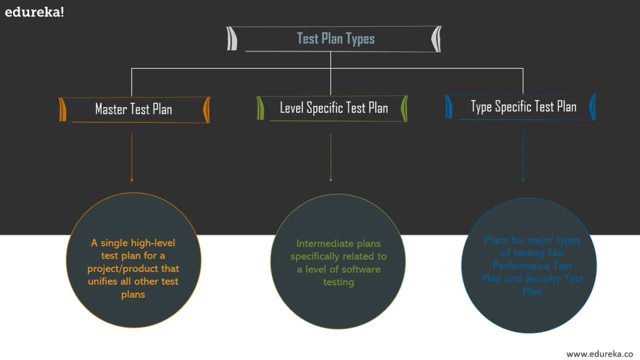 and level specific combined, We call all of them together as master display. So I hope you understand the distinction between different test plans right. moving on, you already know that making a test plan is really important task of test management process. So how do you go ahead and write a test plan? 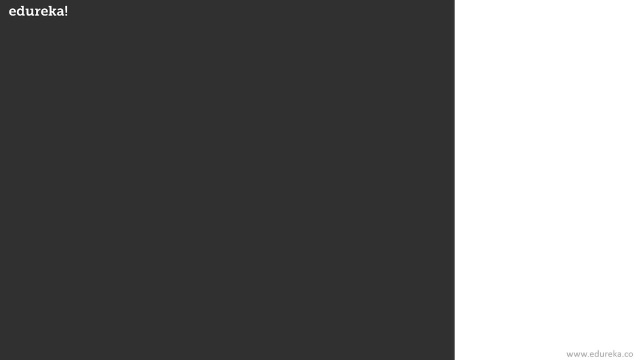 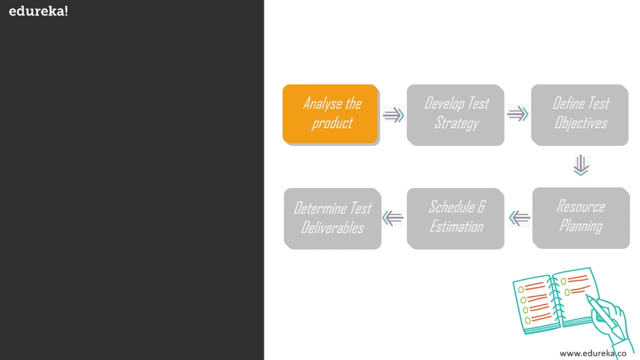 Is that a procedure, or a standard procedure at that? Let's check it out. So, basically, to write a proper test plan, There are six simple steps that you can follow. first step is to analyze the test product. So can you test a product without any information about it? 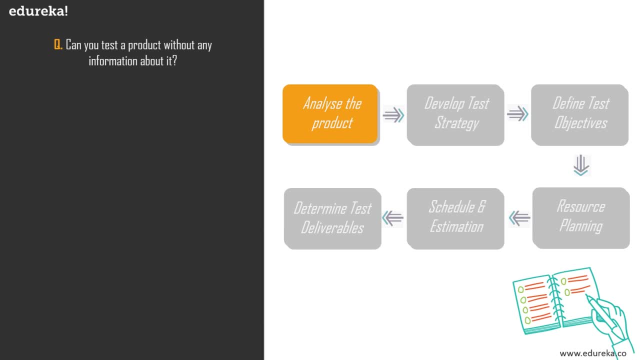 Well, no right. So you must learn a product early and you need to understand the product more deeply before even testing it. So the first step towards creating a test plan is to analyze the products, its features, functionalities, so that you gain deep understanding of the product. further explore the business requirements. 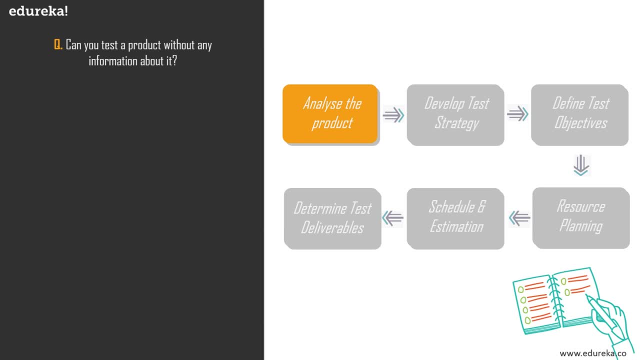 and what the client wants to achieve from the end product, understand the users. use cases to develop the availability of testing the product from users point of view. So basically, at the end it's user who you are trying to impress or satisfy the requirement. So you need to have proper understanding of the product. 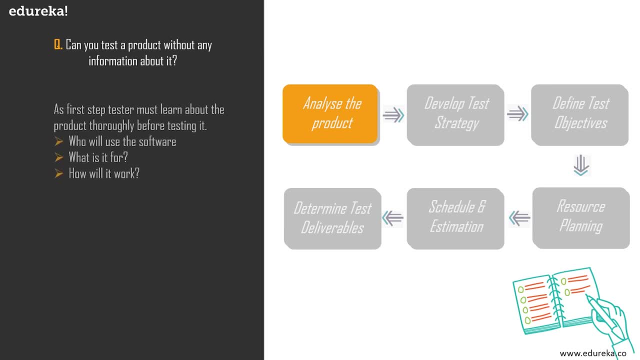 the user requirements and expectations of the product. So how can you actually analyze a product in a systematic way? The first thing is you can go ahead and interview your client designer, developers of the software product, because it's who they start preparing the product from the scratch. 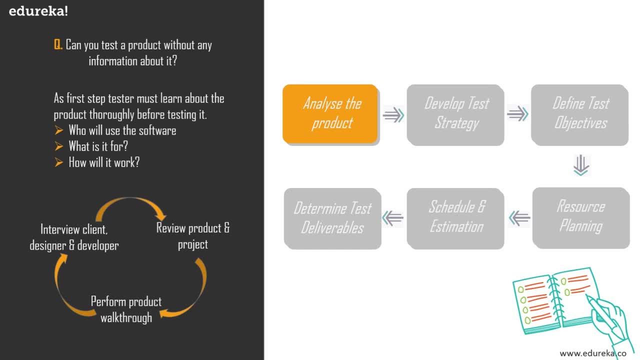 So they'll know more about the product than you do. So go ahead and ask them about each and every minute detail. review the product and entire project Once you get them. don't avoid the important details. go through all the details. Secondly, you perform a product walkthrough. 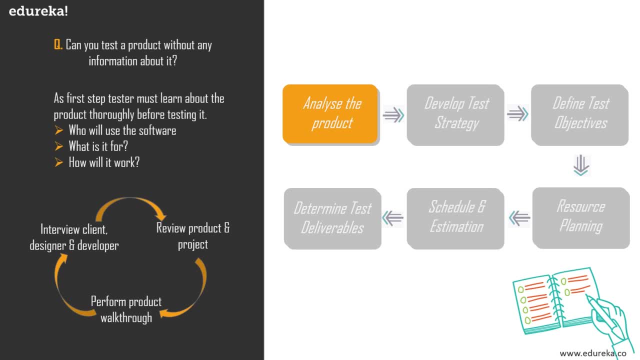 That's nothing, but just use the product as if you are the end user and see if it's as an end user, if it satisfies your requirements or not. So that's how you analyze the product. moving on, The second step is to develop a test strategy. 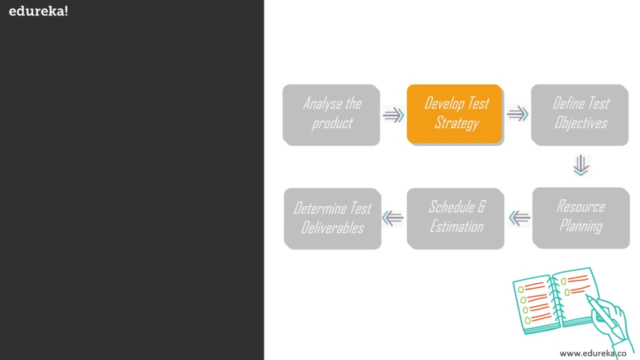 Once you have analyzed the product, you're ready to develop the test strategy for different test levels. So your test strategy can be composed of several testing techniques, keeping in mind test cases and business requirements. You can decide on which type of technique that you want to use. 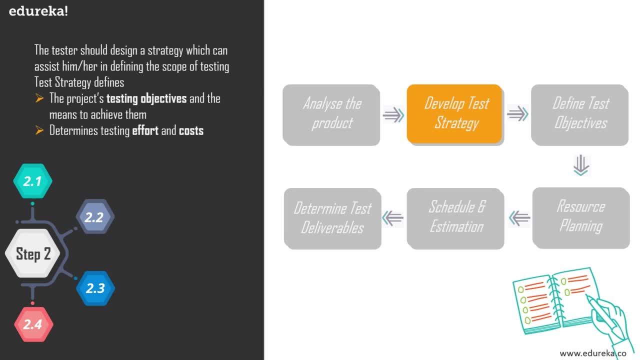 For example, if you're building a website which has thousands of online users, you will include load testing in your test plan. Similarly, if you're working in an e-commerce website which includes online transactions, you will emphasize more on security and penetration testing. 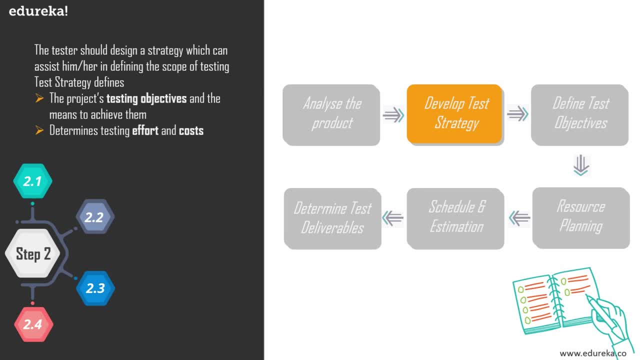 So, depending on your requirement, or actually the user requirements, you decide on the different technique or the strategy that you want to use when you're testing. well, under the step, We do have multiple steps, which is to define the scope, identify the testing type, document the risk. 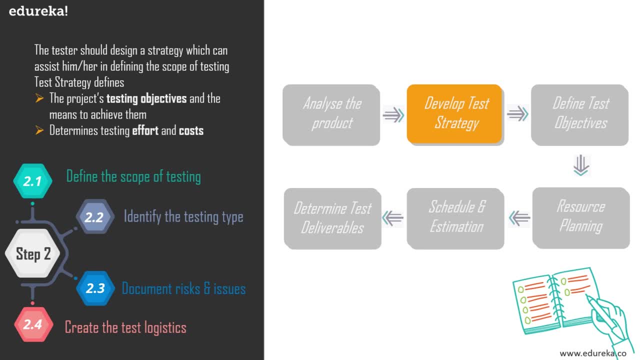 and the issues that you might come across and how to face the risk and all that and, lastly, create the test logistics. Let's not make it more theory based. I hope you've understood the second step. Let's move on to next step, which is to define objectives. 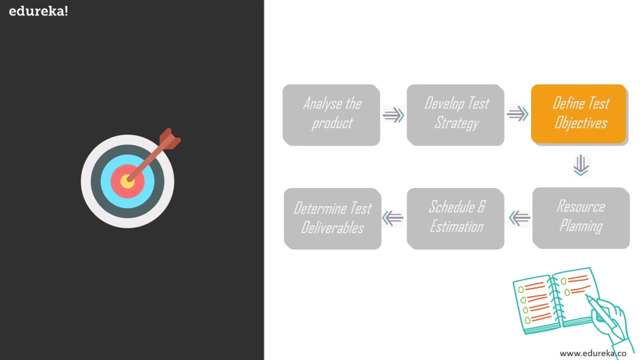 So, basically, a good test plan clearly defines the testing scope and its boundaries. So, as you guys know, the objective of testing is to find as many software defects or bugs as possible, ensure that software and test is bug free before you release it to market. So you need to define a test objective to do that. 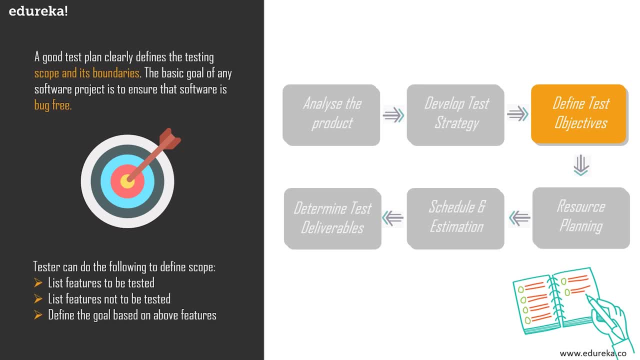 You can just follow two steps, which is to list all the software features. It can be anything: functional, performance, graphical user interface, security, many other things which you might have to test. secondly, after listing all the requirement features, define the target or the goal of the test based on the features. 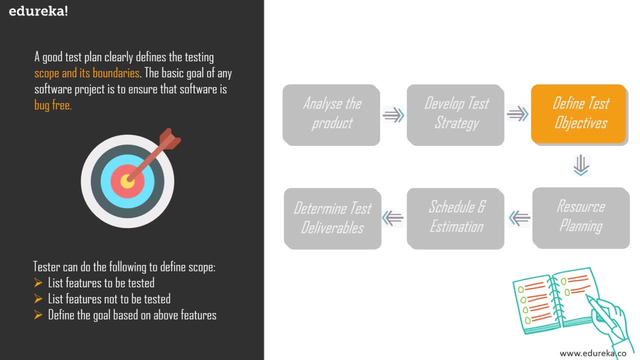 that you have listed down, make a list of features which has to be tested, which need not be tested. This will make your test plan specific and more useful. So, like I said, one of the benefits of test plan is you can avoid your time spending or testing the features which needs to be tested. 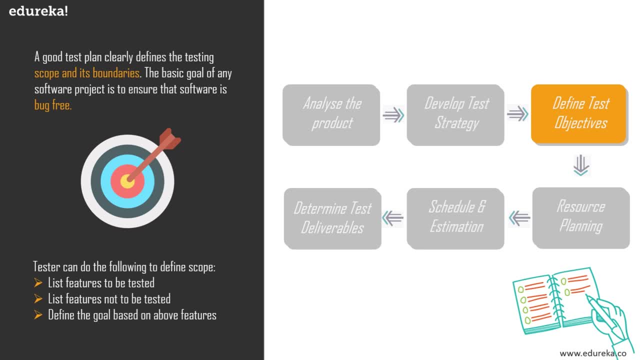 And avoid out-of-scope functionalities, and along with that, you might also have to specify the list of deliverables as output of your testing process. You might need to explicitly Define if any testing techniques, such as security testing, for example, is out of scope for your product. 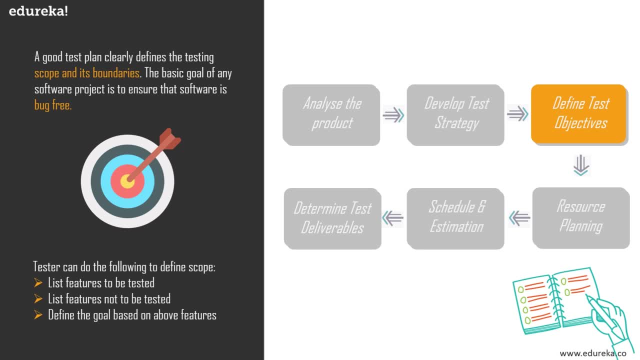 or if you need it or if you don't need it. all such things come under defining test objectives. moving on to next step, We have something called resource planning. Obviously, when you're testing, you need a lot of resources, tools, people and all that. so resource plan is a detailed summary. 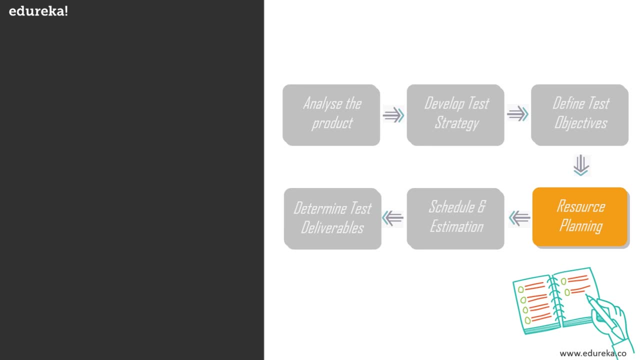 of all types of resources required to complete a project task. It could be human, Like I said earlier, equipment materials needed to complete testing project. It's an important factor of test planning because it helps in determining the number of resources. It could be employment equipment, anything to be used. 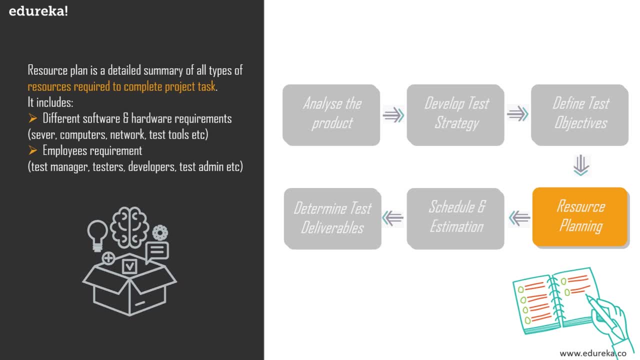 for the project. Therefore, the test manager can make the current schedule and estimation for that particular project. Well, I'm not going to list down all the roles and responsibilities or the people involved in all that, but to understand the step, It's nothing. 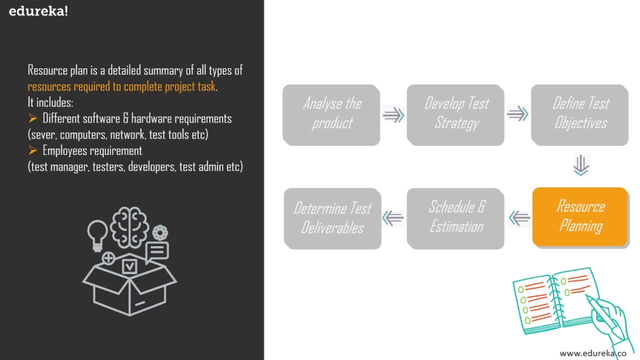 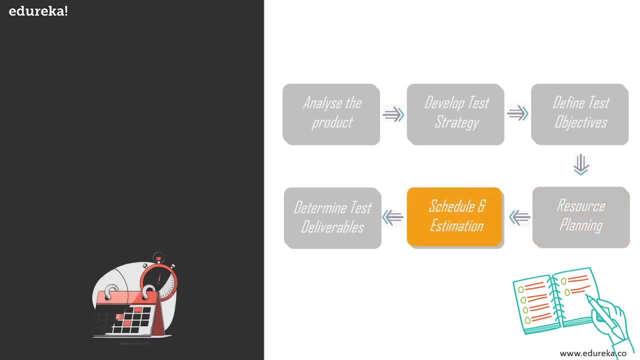 It's just planning about the resources which you might require when you're actually testing. the next step is schedule and estimation. So, with the knowledge of testing strategy and scope in hand, you're able to develop schedule for testing. So divide the work into testing activities. 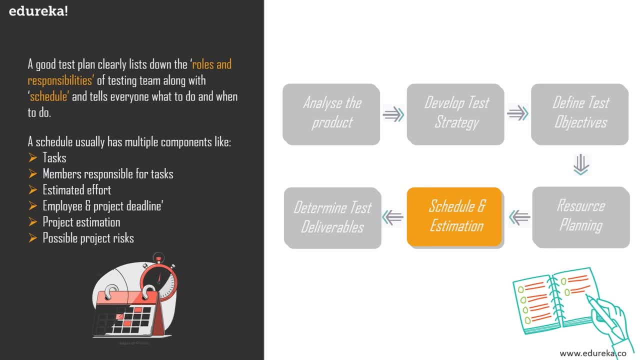 and estimate the required effort. You can also estimate the required resources for each task. So make a table. It's simple. right in one column You can have the list of testing activities. in second column You can have the members who are responsible for performing those activities. 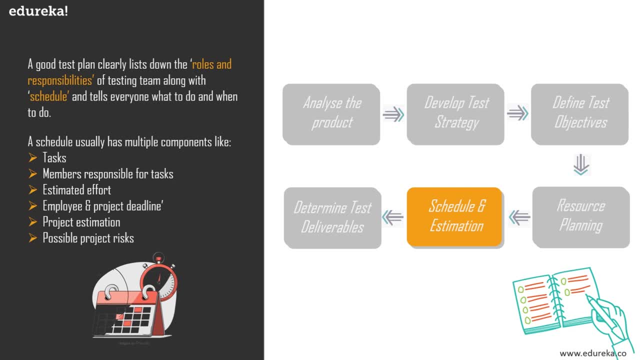 and then you might actually include the schedule as well as in when this task has to be completed, by when is the deadline? and all that you can also include under the column which says what resources are required to complete the task, So that way you can control the progress. 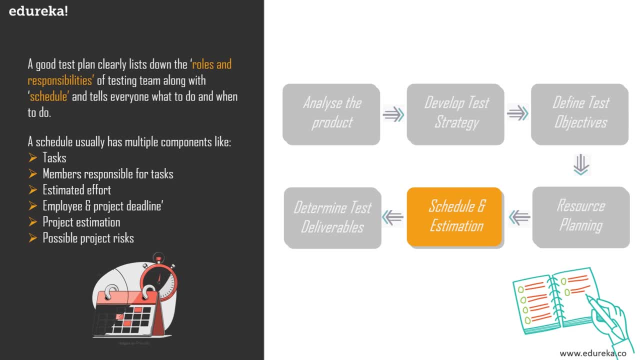 or of your testing process. So to create the project schedule, the test manager needs several types of inputs, like we discussed about deadline estimation, risk and many other details. So a good test plan clearly list down So rules and responsibility of testing team, as well as the team manager as well. 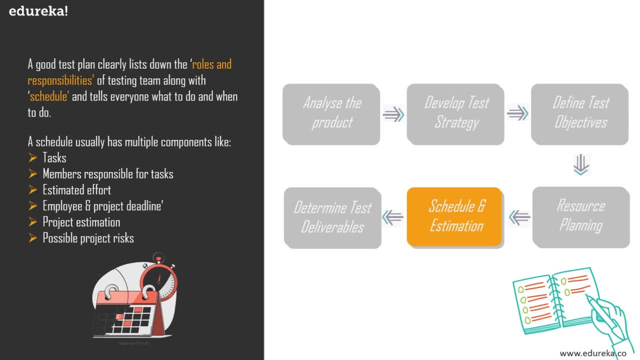 So, basically, the table which you've created, which you should create, will tell everyone what to do, when to do and what are the risks that might they might come across, and all that. and last step is to determine test deliverables. So test deliverables is basically a list of all the documents. 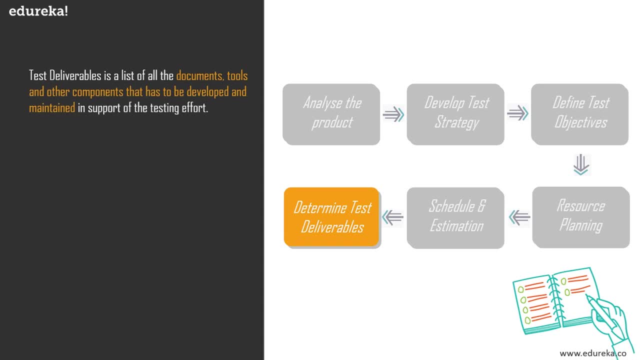 tools and other components that has to be developed and maintained in support of the testing effort. There are different test deliverables at each phase of software development, like cycle. So basically you can divide the entire software testing into three parts: before testing, during testing and after testing. 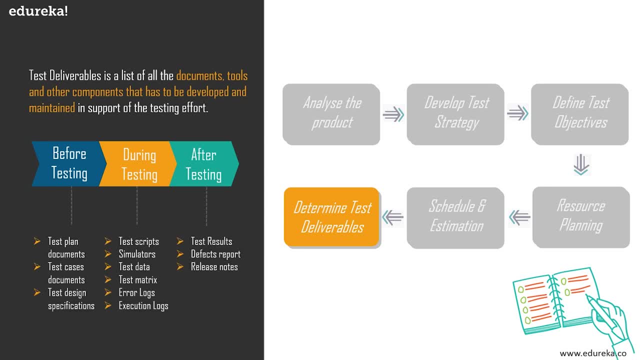 and during this three phases of testing, you do have different test deliverables. For example, before testing, you might need something regarding test plan document, test case document, test design specifications. There's all before you actually even begin testing. then, during testing, you need something like test scripts, test cases. 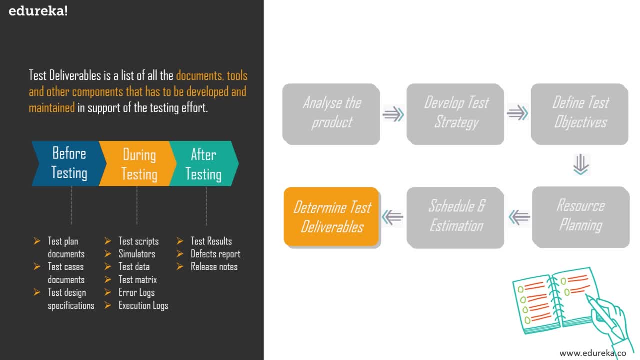 simulators, test data matrix, error logs, execution logs and many other things. similarly, after testing, you might need to create reports, defect reports, release notes, issues regarding the risk that you have faced and how did you overcome and all that. so these are nothing but test deliverables. 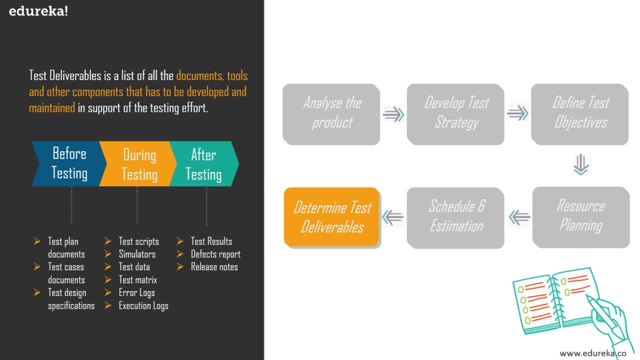 Well, these are the six simple steps that you should follow. but, lastly, your test plan is incomplete without anticipated risk mitigation techniques and risk responses. Well, there are several types of risk in software testing, such as schedule, budget, expertise, knowledge, So you need to list down the risk for your project, along with 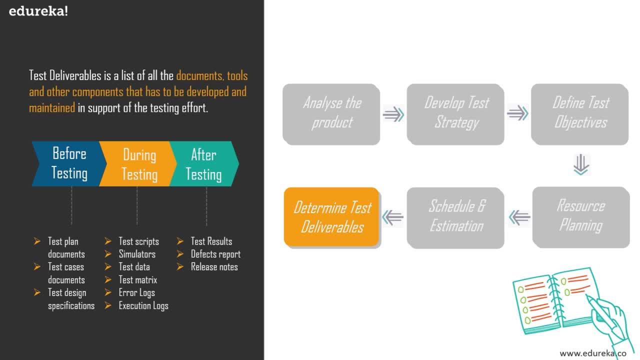 the risk responses And the mitigation techniques to lessen their intensity. So that's how we write a test plan, guys. It's easy, right? You analyze the product. after that you develop a test strategy, decide on the type of testing that you want to do, then define. 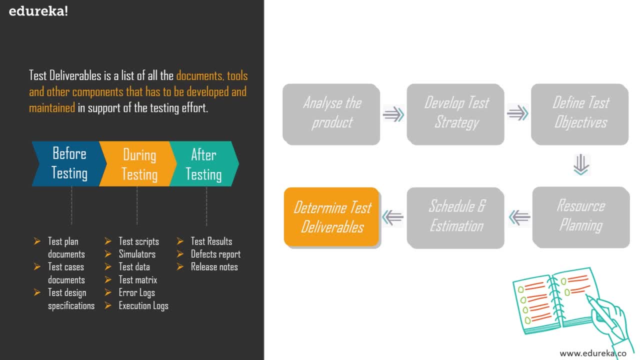 your objective as invite You actually want to test, then estimate the amount of resources that you might have to require or that you might require by performing testing. then do think about your dual and estimation like that as a point in your test plan And, lastly, determine the test deliverables. 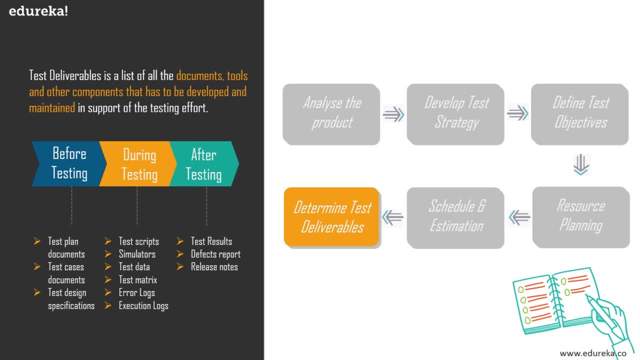 Well, it sounds easy, But what do you actually include in a plan? different people may come up with different sections to be included in testing plan, but who will decide what is the right format? Well, you can go for it to please. standard test plan template. 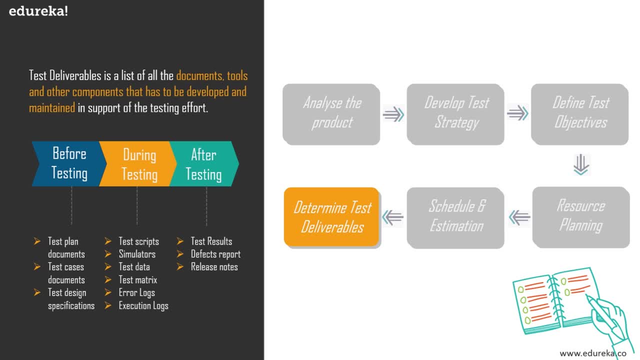 to assure that your test plan meets all the necessary requirements. Well, anybody just can't go and write test plan according to their requirements, right? It messes up. So there's a standard format, which is created by IEEE, that you can write or you can use to write your test plan. 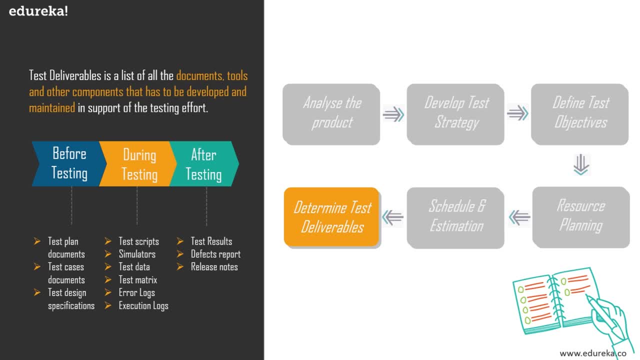 Now, if you're wondering what an IEEE is, it's an international Institute that defines standards and template documents which are globally recognized, so you can use the standard template to write your test plan. It has defined IEEE 829 standard for system and software documentation, 829.. 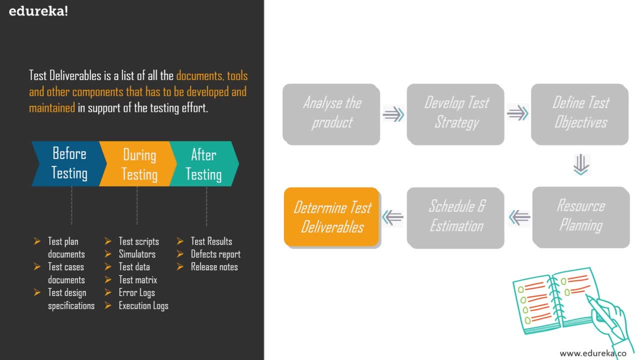 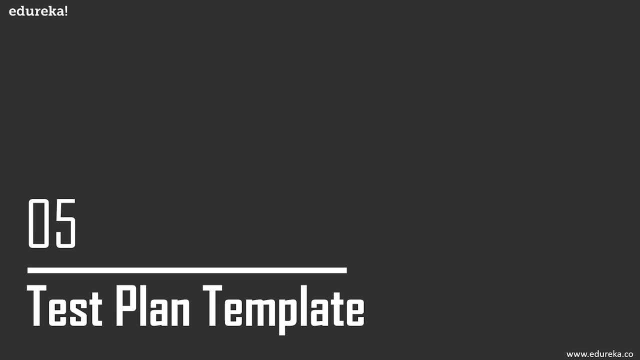 It specifies the format of set of documents that are required in each stage of software testing. So let's briefly discuss What are the things that you should include in your template. I won't make it much theory based. I'm just going to mention the parameter. 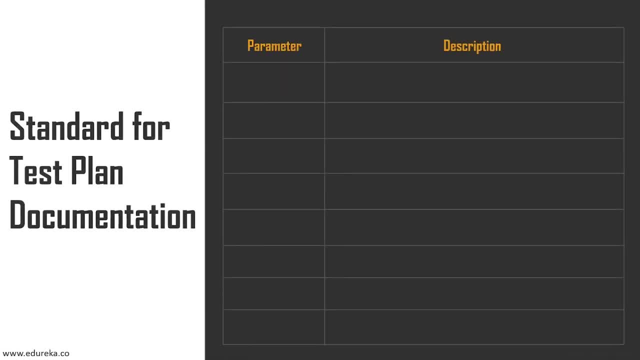 and what does it actually have to include? So let's start. So the first parameter is test plan identifier. So, as a name actually suggest, it uniquely identifies the test plan, it identifies a project and it may include version information as well. It also contains information of test plan type, the types. 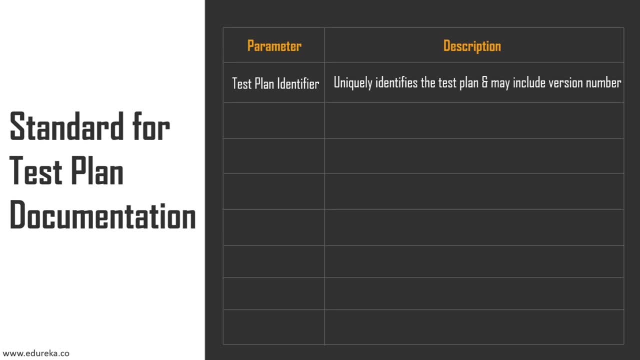 that we discussed earlier: master test plan, test level- specific test plan and testing type- specific test plan. So that's all basically a one. look at this plan identifier. You need to know what testing is done, What are you going to test. and all that, then an introduction. 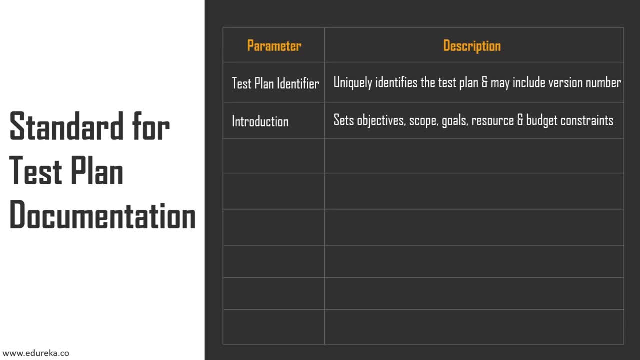 it contains a summary of entire test plan. It sets the objective, scope, goals and many other things of test plan. It also contains resources budget constraints. It will also specify any constraints and limitations of a particular test plan. coming up next is test items. It's a software item that is application, which is under test. 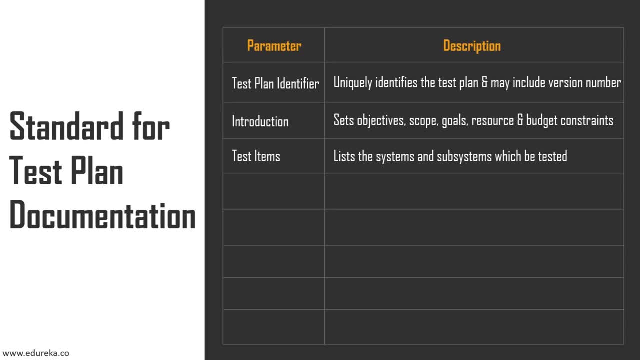 this parameter list the test items, such as software products and their versions and all that and next you have features to be listed in the section. all the features and functionalities which need to be tested are listed there in very detail. It should also contain differences to requirements specification. 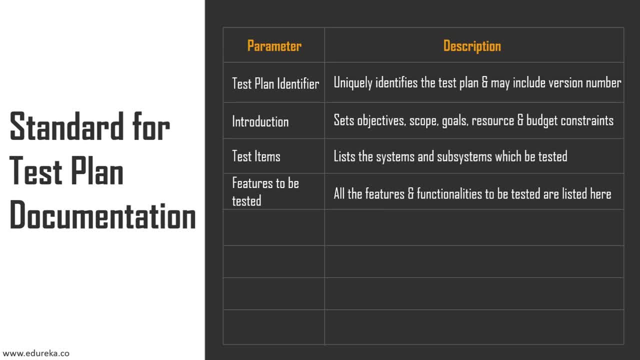 documents that contains details of features which need to be tested. So, basically, it contains all the features and the links to the features which need to be tested. Obviously, since we have features to be tested, We also have a parameter which says features not to be tested. 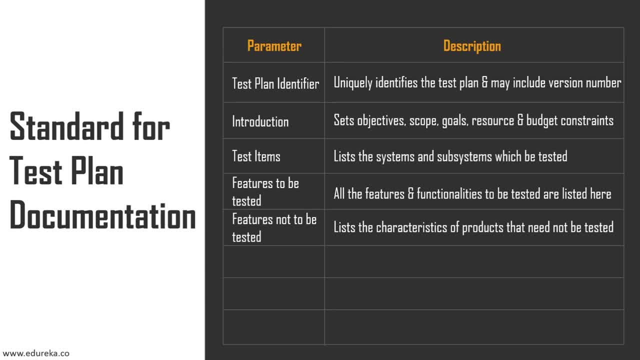 It basically lists the characteristics or the products or the features of the product that need not be tested, or you can say, out of scope. It also contains the reasons as to why this feature should not be tested, and then you have something called approach. in this section, approach for testing will be defined. 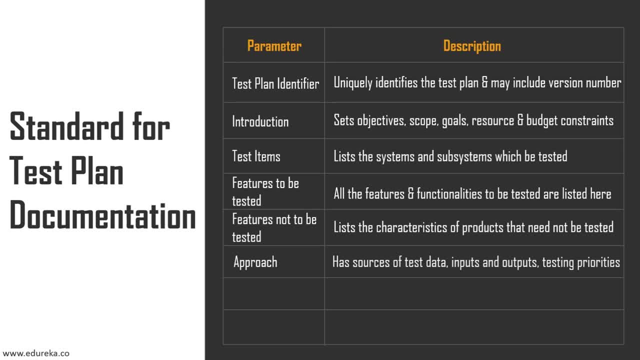 It contains details of how testing will be performed. It contains information of the sources of test data, inputs, outpost testing techniques and priorities. It will define the guideline for requirement analysis, develop scenarios, derive acceptance criteria, construct and execute test cases and many other things. and then you have something called item pass or fail. 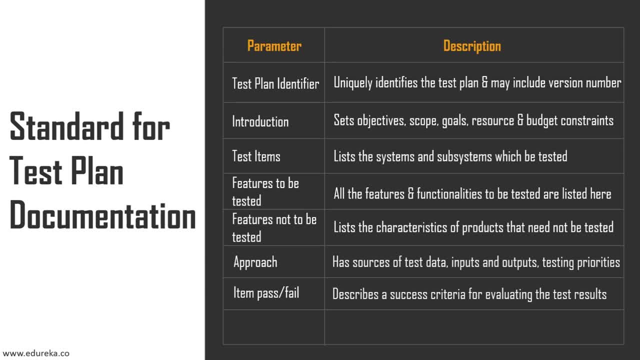 as you can see it straightforward, It describes a success criteria for evaluating your test results, Basically documents whether a software item has passed or failed the test and based on what you should decide. if it has passed or failed the test, then you have something called suspension criteria. 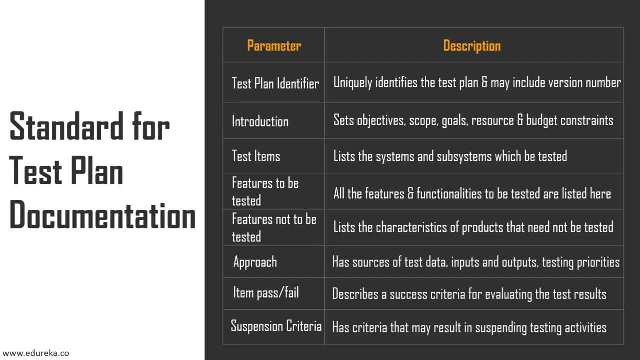 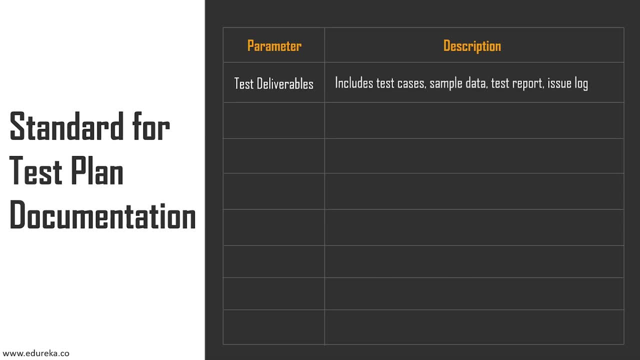 It will describe any criteria that may result in suspending the testing activities and subsequently the requirements to resume the testing process. Then you have test deliverables. We did discuss the different things that you might require during three stages of testing, that's, before testing, during 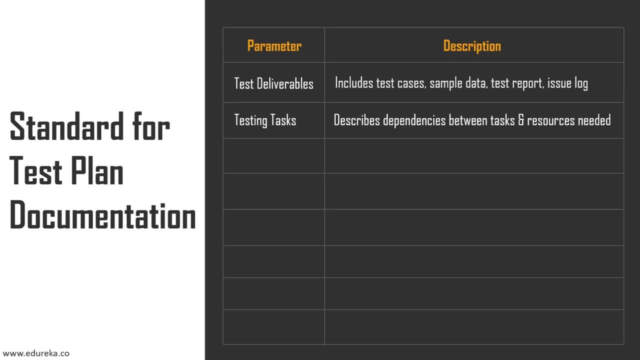 testing and after testing and all that. then you have testing task. In this session, testing tasks are defined. it also describes the dependencies between any task, resources required and estimated completion time for these tasks. testing task may actually include creating test scenarios or creating test cases, creating test scripts, executing these. 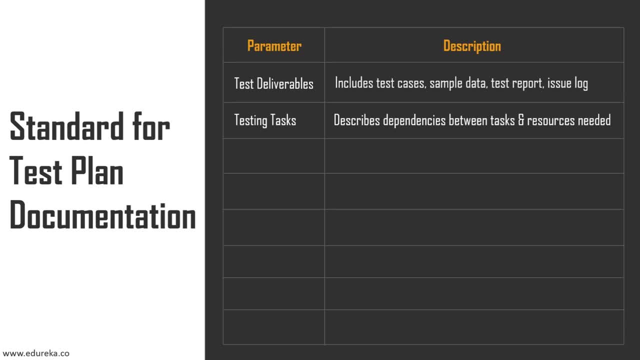 test cases and scripts, reporting bugs, creating issue logs and many other things. basically, the tasks that you want to perform while testing are all come under this testing task. Then you have environmental needs. So this section describes the requirements for test environment. It includes hardware, software, any other environment requirement. 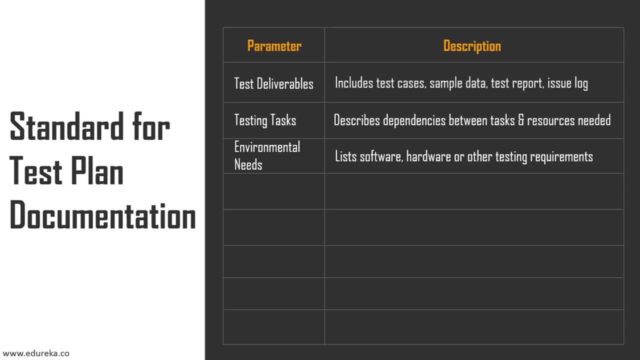 for testing. So the plan should identify which testing equipment is already present, what needs to be newly brought, and all that. moving on, We have something called roles and responsibilities. Obviously, when you're performing testing, you have a lot of people in your team, So you need to define the rules and responsibilities of each. 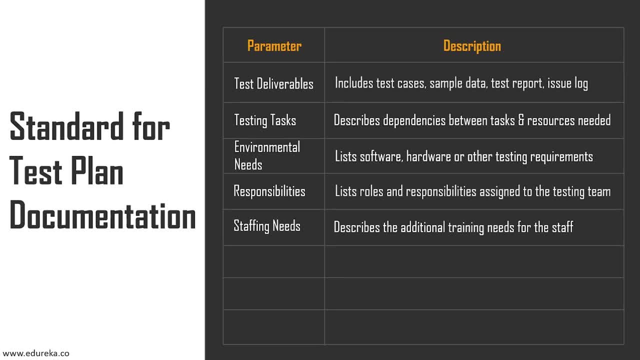 person involved. That's what you do in this parameter. Then you have staffing needs. it basically describes the training needs Of the staff for carrying out the plant testing activities successfully. Well, if they need, they can be further trained on before moving on or before putting them on to next level of testing. then you 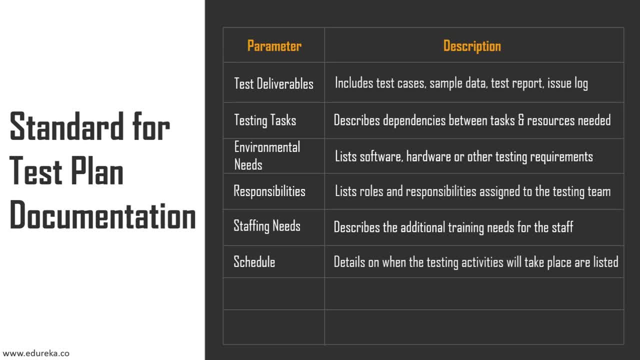 have something called schedule, So you provide a summary of the schedule, specify key test milestones, or you provide a link to the detail schedule and all that. the schedule is created by assigning dates to the testing activities. You can prepare a detailed table, like we discussed earlier. 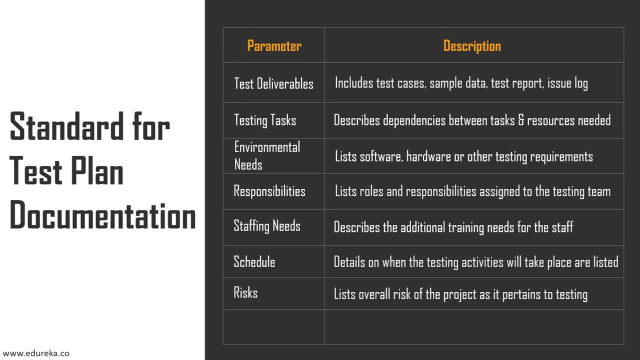 and then obviously the risk. risk play a very important role. You have different risk regarding security, Bugs and many other fields, So you'll start risk and how to mitigate them, And what? how does that risk actually affect your testing and all the details here. 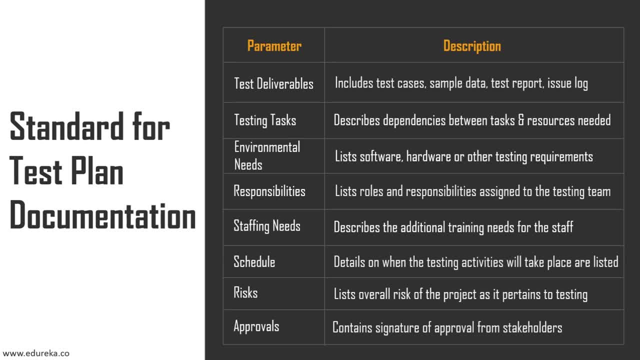 And finally, you have approval. this section basically contains the signature of approval from your stakeholders that your test plan is perfect and you can proceed to testing. So I hope it wasn't very difficult to understand, right? it's straightforward. You can actually understand by just looking at the names of. 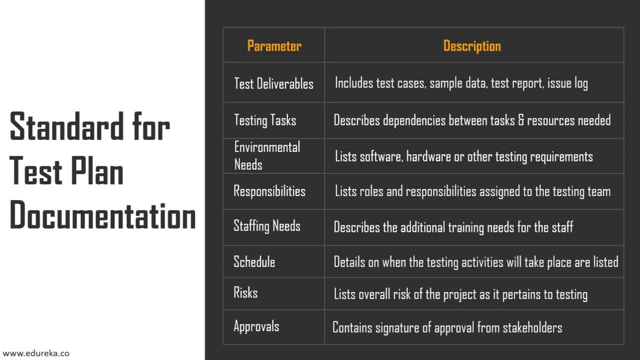 the parameters really straightforward, So please do go through it again If you're found Found that the theory part was more. the slide should help you out here. So that's it, guys. with this We have reached the end of the session. We discussed the details of the test plan and what to include. 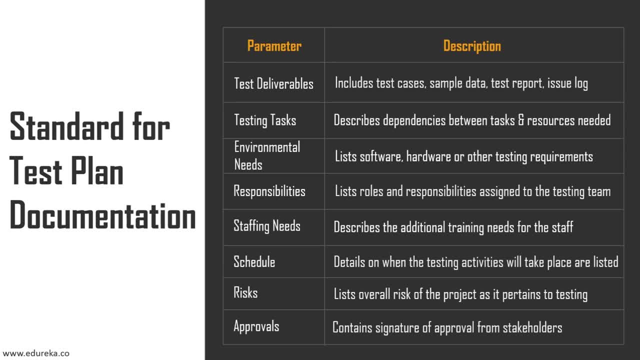 in a test plan. Basically, a test plan is a guidebook for testing process and it's vital to keep testing process on right track. So, basically, you can use a test plan as a mechanism to see conscious, to drive information exchange and consensus, and to prepare yourself for further rounds of testing. make it. 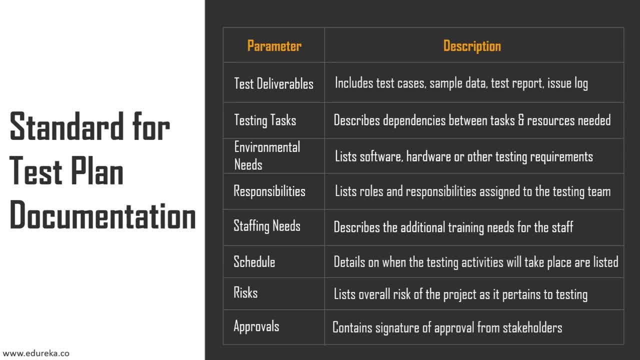 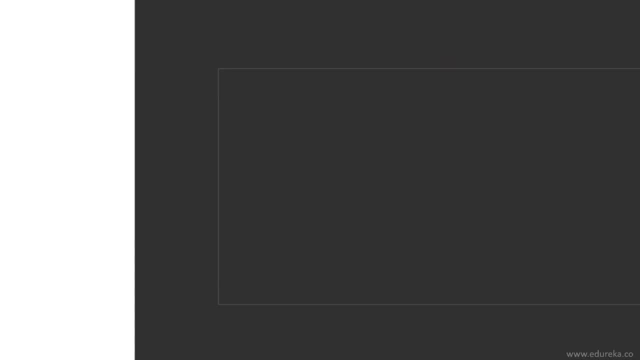 valuable for you and your stakeholders. Make your test plan work for you and not against you. So the main aim of the test plan is to make testing much more easier for you. So that's it, guys. I hope the session was informative. If you have liked the session, please do click on the like. 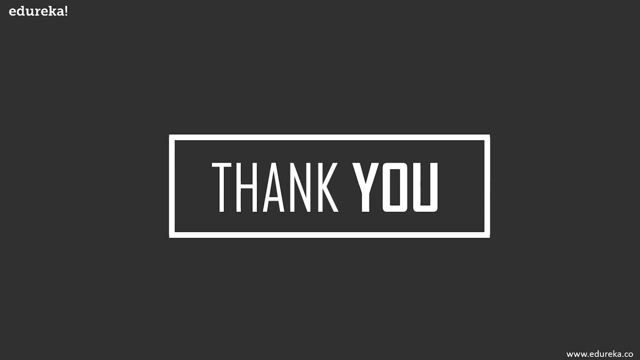 button, and if you have any queries or doubts, you can put them in the comment section below and we will get back to you as soon as possible. and please do not forget to subscribe edureka YouTube channel If you want to know more about other trending Technologies.